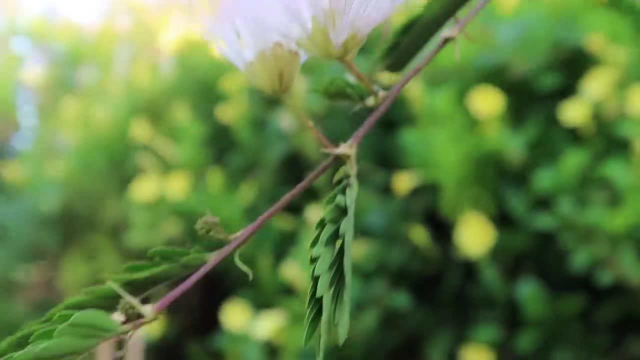 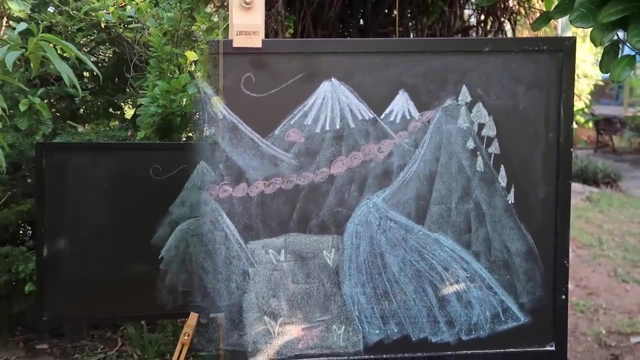 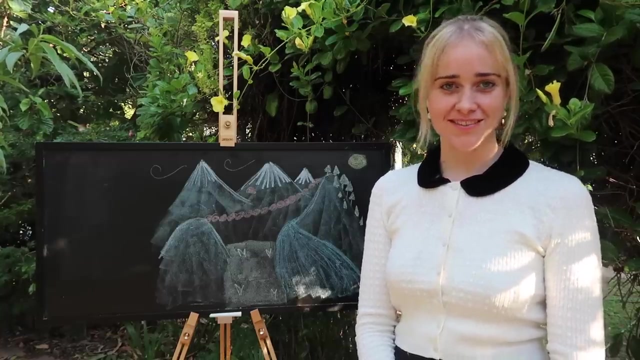 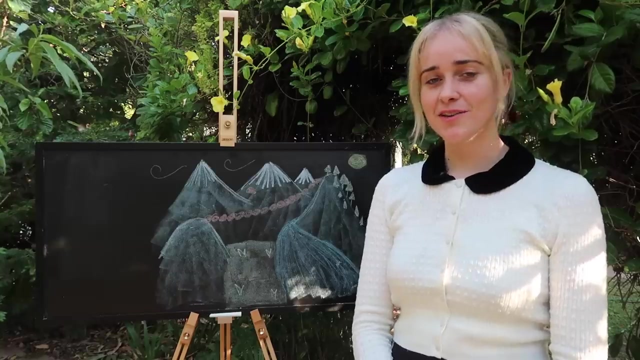 Hi, I'm Toby and welcome to another episode of The Joys of Mathematics. Today I'm not going to throw any formula or equations at you. I'm just going to tell you a story Now. behind the story, you might be able to find, hidden away in there, the essence or some of the intuition behind calculus. 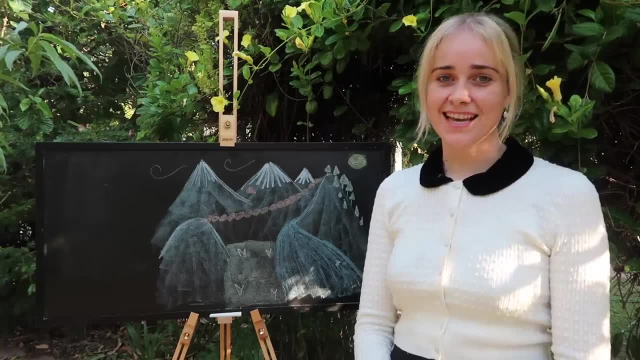 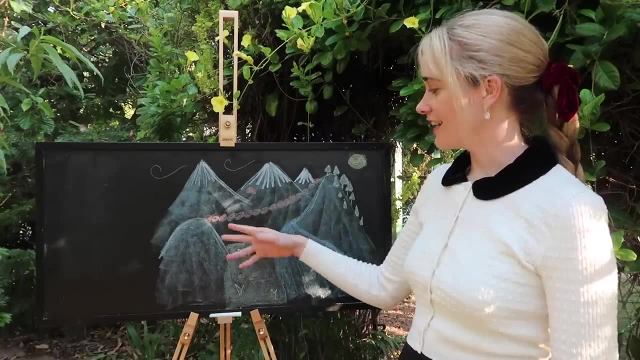 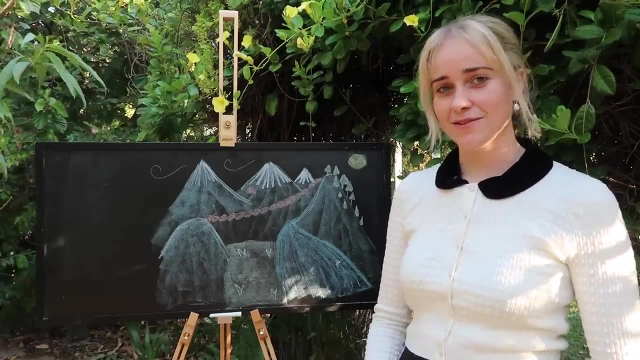 but don't worry, because this is not going to be a mathematical story. this is going to be a story about a guy called Bob who lives in a little hut in some snowy mountains. So I want you to just sit back and relax and enjoy listening to the story. Don't stress too much about trying to turn your 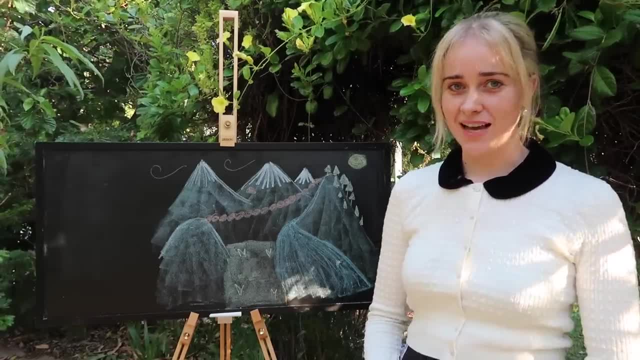 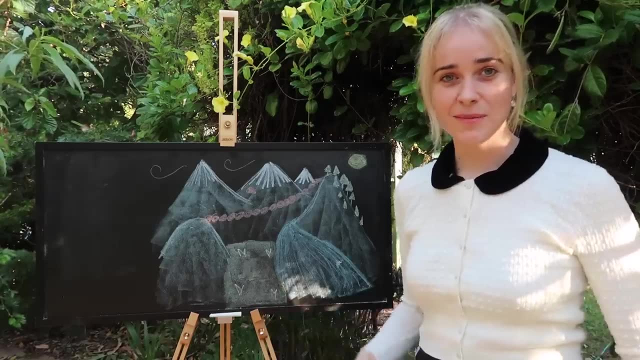 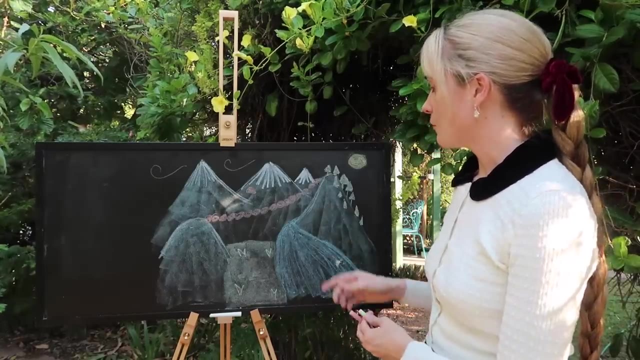 brain on, but hopefully you might learn something along the way. So, like I said, this story is set in the mountains. Now it's a very windy and stormy day in the mountains. we've got a lot of wind. A couple of things happen, though, which are not ideal. The first one is that one of the trees 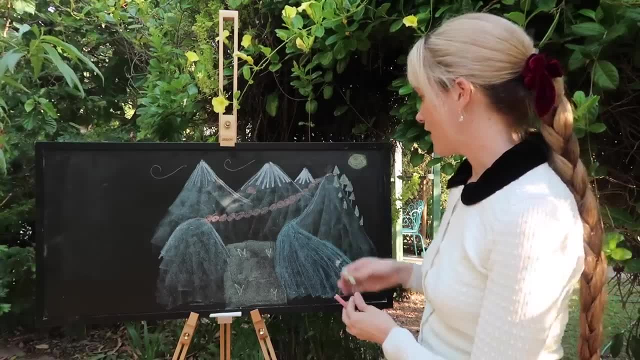 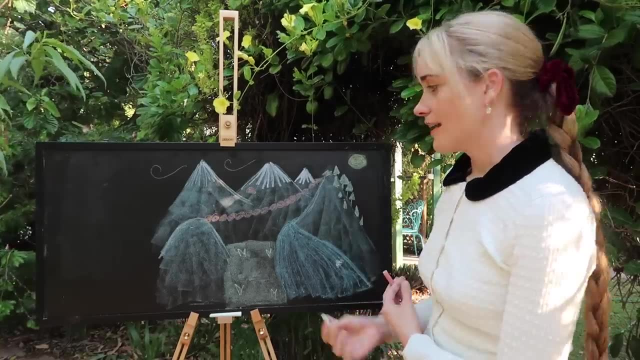 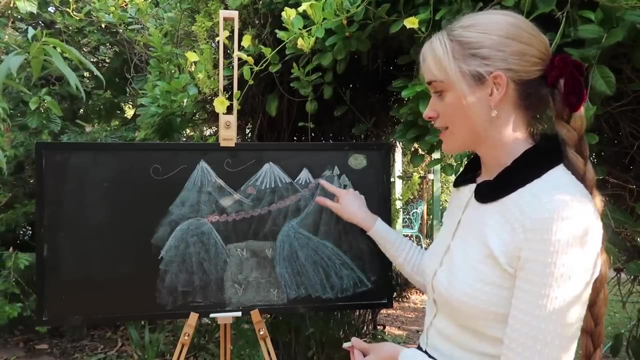 one of these little happy trees on the mountain over here is blown over and it falls. Not such a happy little tree now. The second thing that happens in the windstorm is that a little section of the bridge which is made of logs here and connects one hill to another over a river. 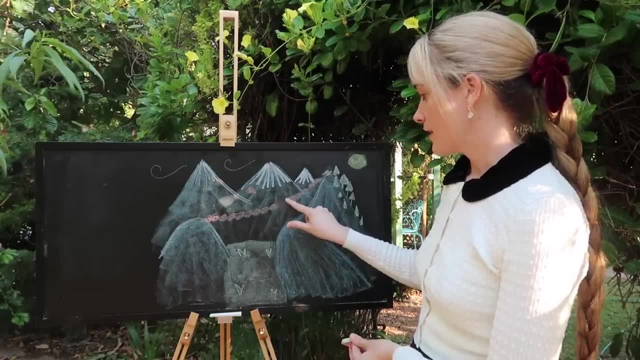 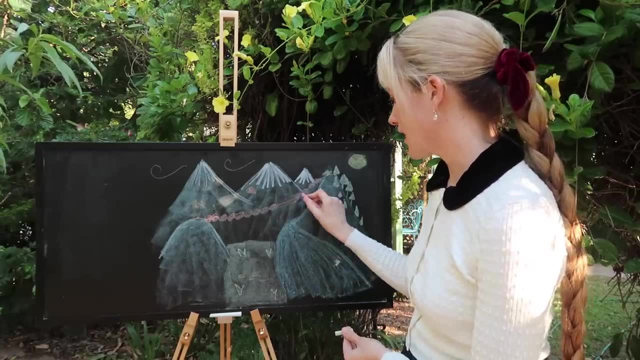 it breaks away and falls. What it's left in its place is just a couple of wires that used to hold the logs together. The logs that have broken off don't fall straight down into the river. they just fall down into the river. So it's just a couple of wires that used to hold the logs together. The logs that have broken off don't fall straight down into the river. 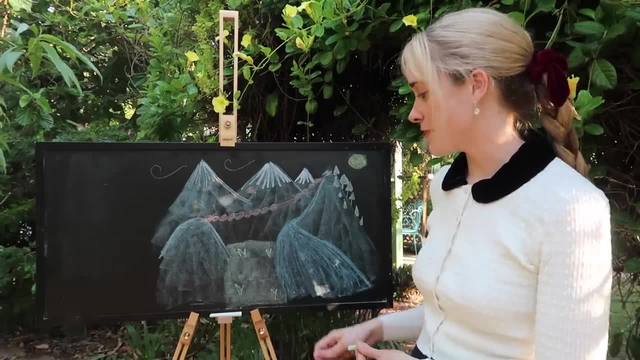 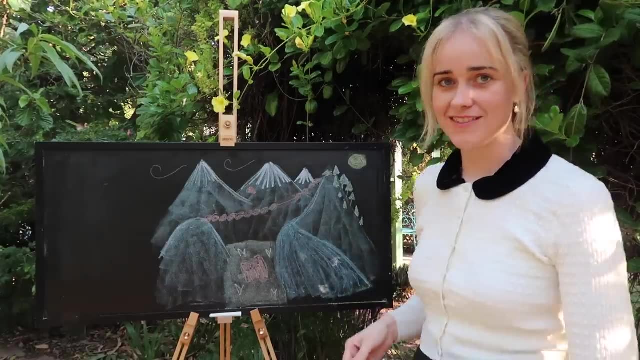 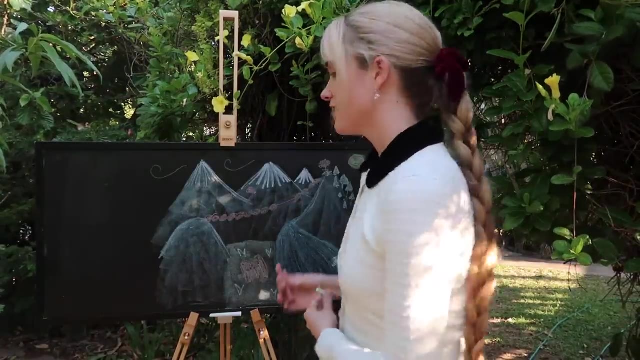 but they are blown sideways a little bit to this grassy meadow down here. Okay, so all of this goings-on sort of concerns Bob, who lives in his little hut and he comes out to check that everything is okay. Let's draw Bob here Now. this story is about the lengths that Bob goes. 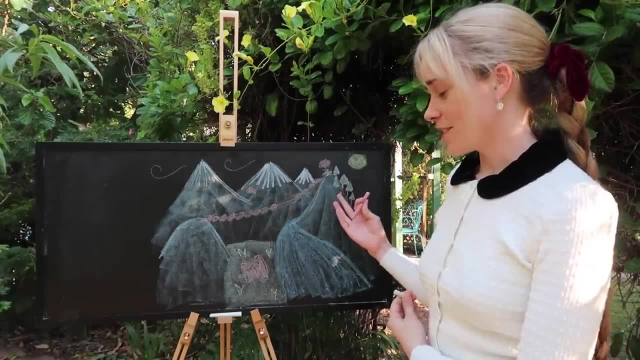 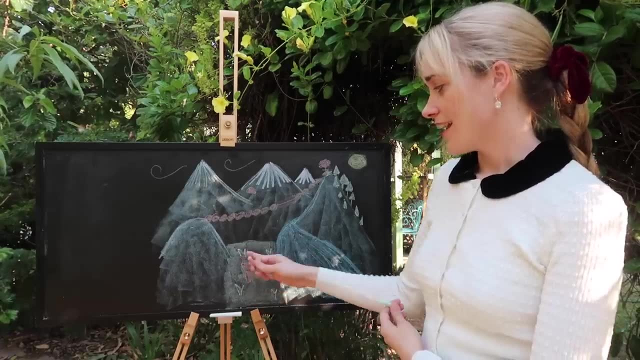 through to do the right thing. Now, the reason he's so concerned and that he comes out of his hut is he knows that down here, in the meadow where the wood has fallen this meadow, are a couple of deer who are very dear to him. They're a. 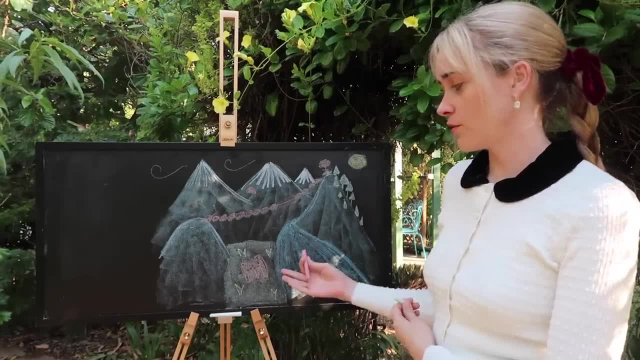 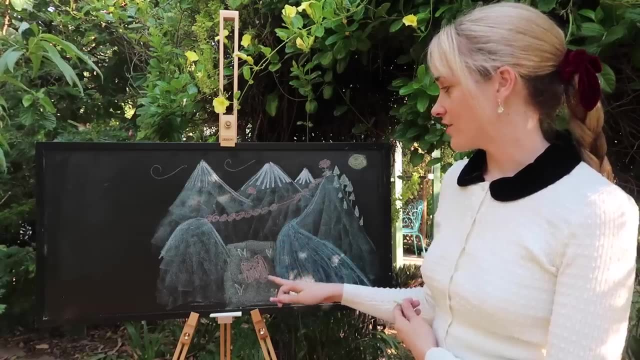 couple of friends of his and he's concerned. He wants to make sure that everything is alright and that no one's been hurt and down in this meadow- Now to be able to get down there and check, he's going to have to cross this bridge of. 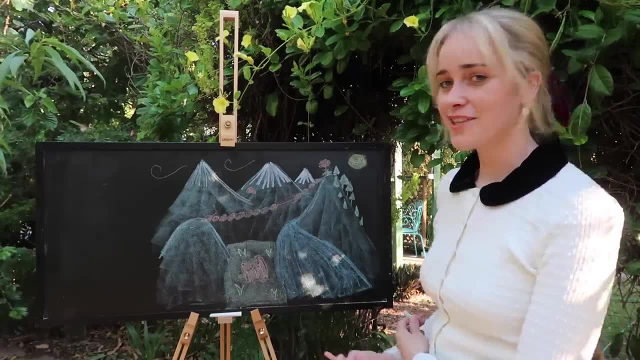 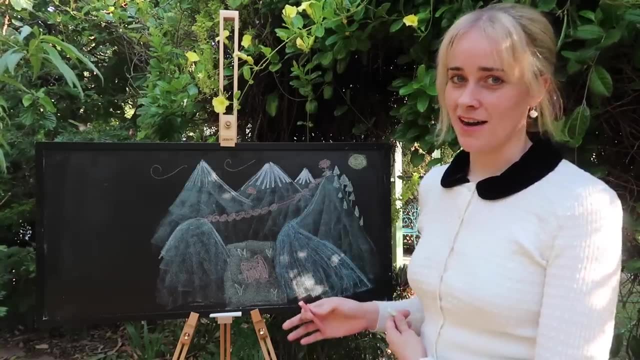 logs. Now, obviously the problem with that is that a section of the bridge is missing. Bob's gonna have to come up with a plan. He does have one idea in mind, And that is that, looking at one of these fallen trees beside him on the hill, he 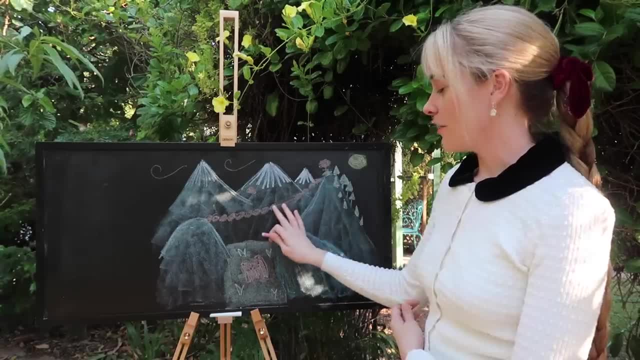 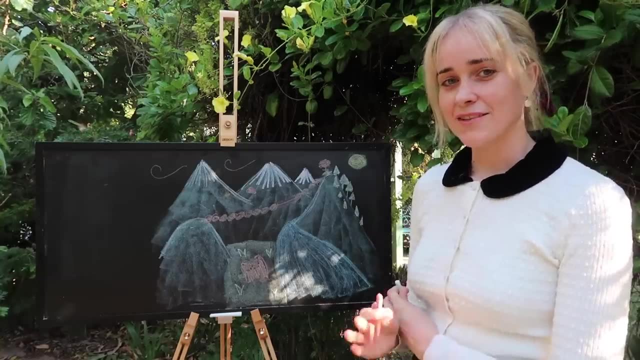 thinks he might be able to use that tree, lay it down along the wire that's left in place on the bridge and create a little ramp for himself to walk down. Now there's only one problem that Bob really needs to consider about this plan, and 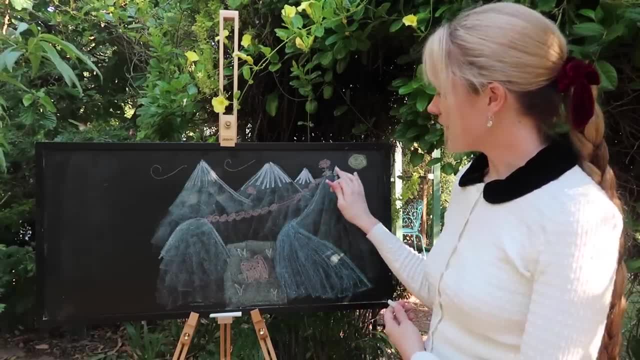 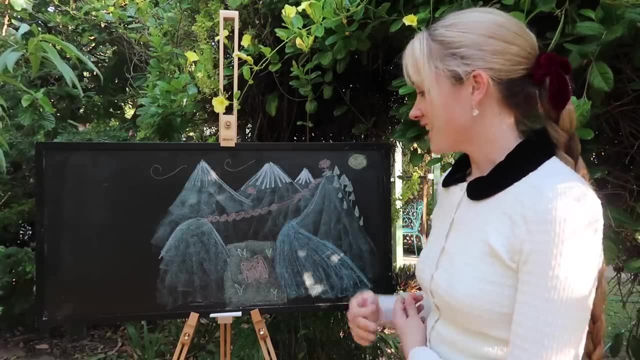 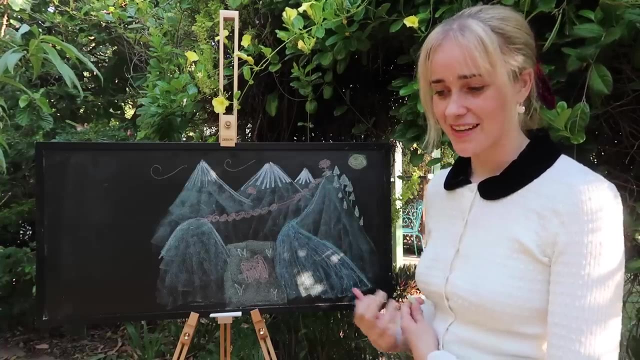 that is that you know we've got a curved bridge and if we lay a flat tree down on this wire, that part of the bridge there is going to go straight, And he doesn't want it to end up being so steep that he just slides down it and isn't able to climb back up to get home. You know, Bob has. 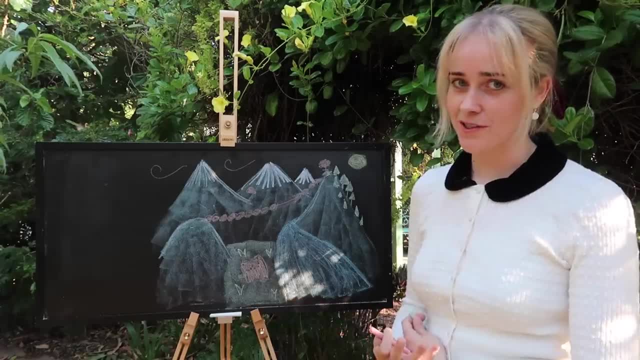 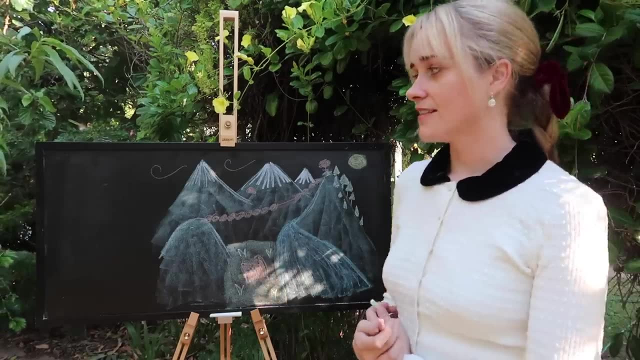 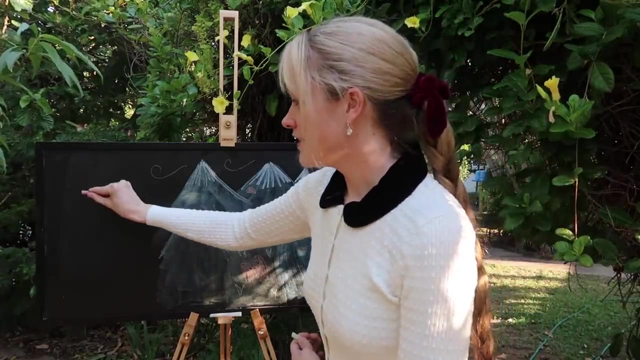 also some very old shoes that are completely worn away on the bottom, so he doesn't have much friction coming from his shoes. One thing that Bob knows from past experience is what kind of slopes and ramps he is able to walk up with these shoes of his, Now, obviously walking along flat ground. 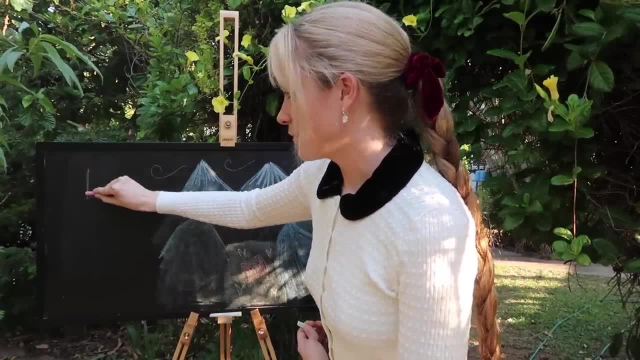 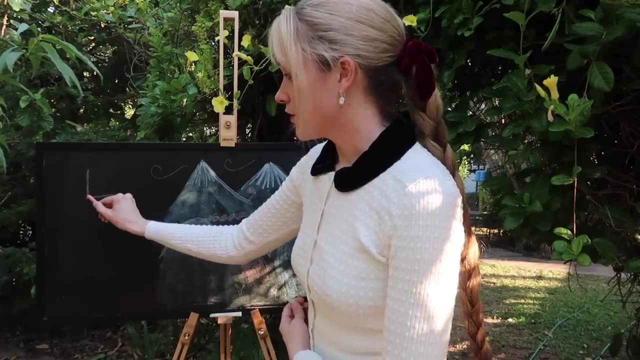 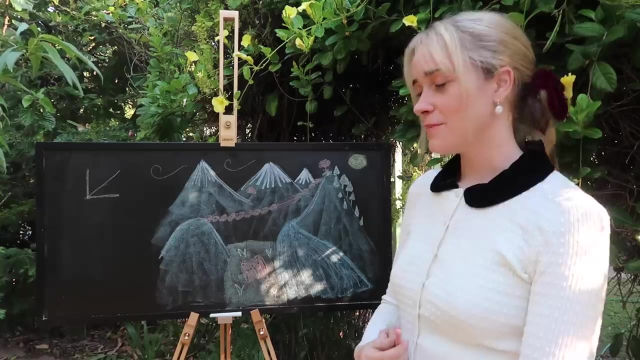 is going to be easy. walking straight up and down a wall is going to be impossible. but what Bob does know is that, exactly in between vertical and horizontal, if I were to draw a line exactly in between them there, that is the limit of how steep a ramp Bob can walk up with his shoes without slipping. 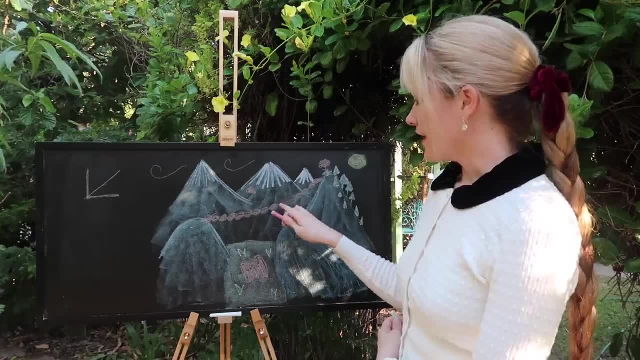 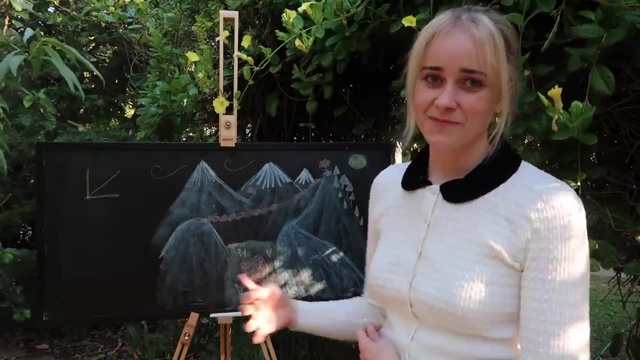 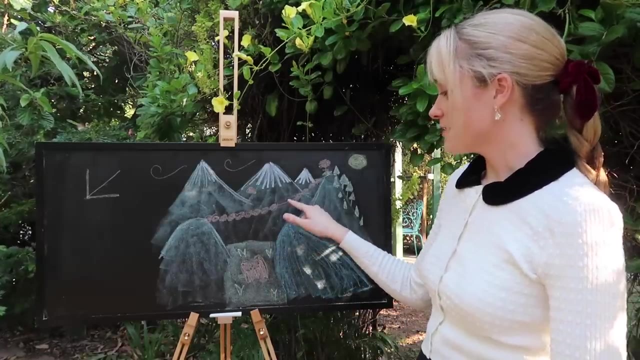 Okay. so if we know that this little flat tree lying down here on the ramp is going to be as steep as that ramp gets up, as this or less, it'll be fine, there'll be no problem. So Bob needs to check and the way that he's going to measure how steep the little tree ramp would be once. 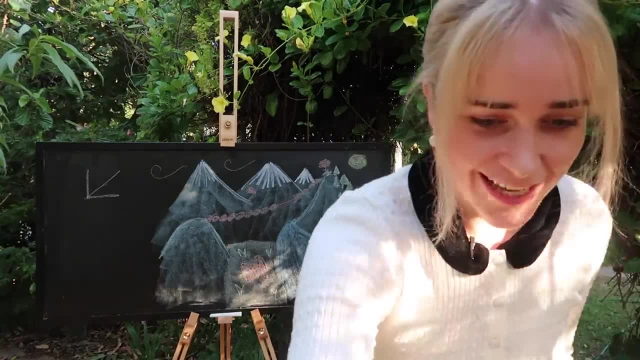 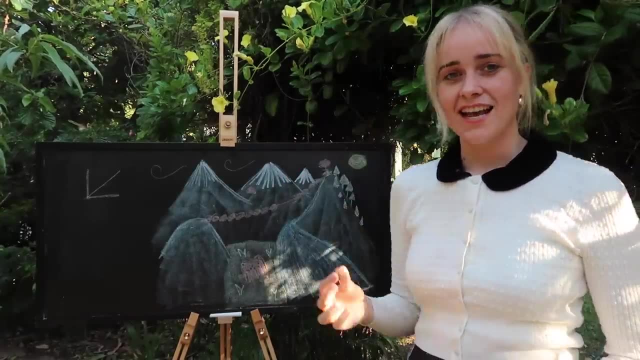 it's on the bridge is that he picks up a pebble- Now I've got one here by the camera- and he holds the pebble to his eye and he looks at the hole in the bridge and he just uses the pebble to measure as sort of a measuring stick. how 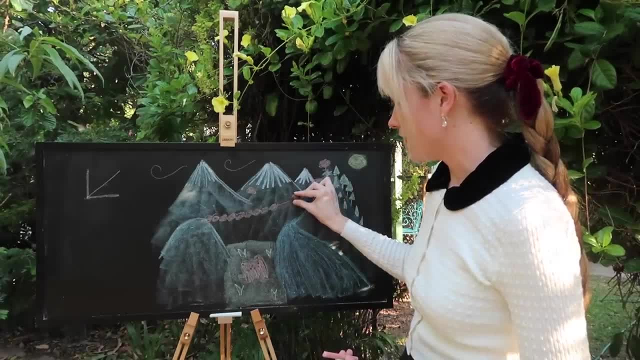 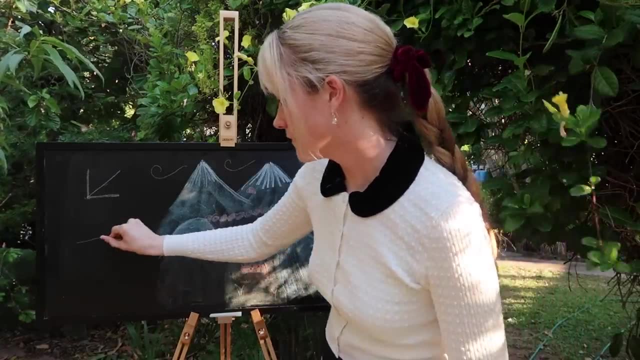 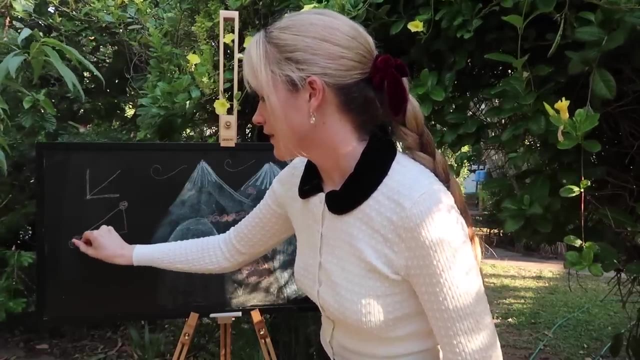 many pebbles he think could fit in the area vertically between the missing logs. So if we had a little triangle. this is one log, this is the other log. these are the missing logs that would have fit in along here and this is the wire that's. 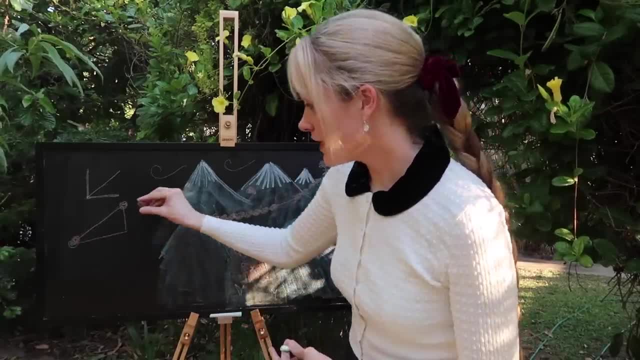 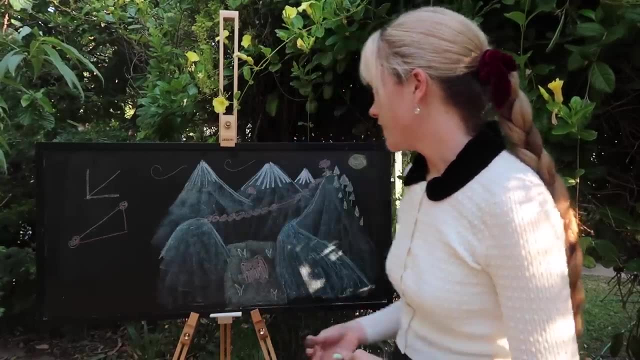 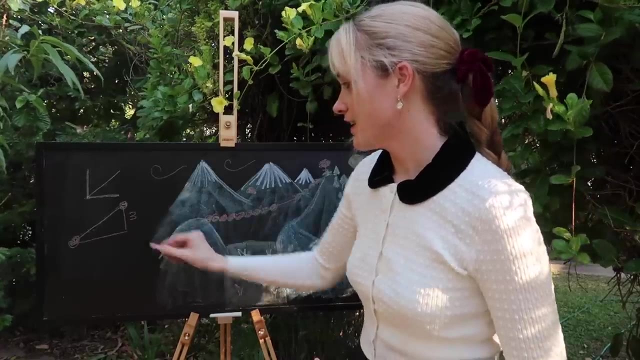 just in their place, holding them together, He measures how many pebbles he thinks with his eye could fit down here and how many could fit across here. Now what Bob measures, just by using his little pebbles, is that he thinks he could fit three pebbles in this height and three. 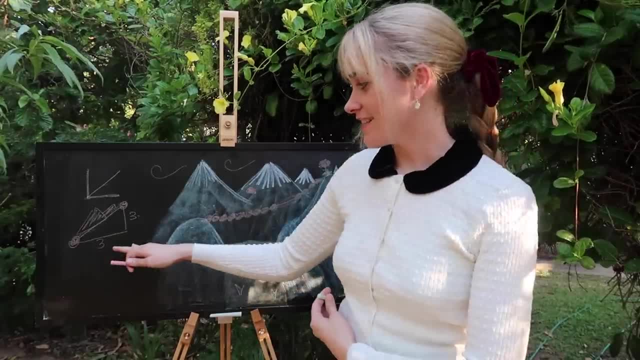 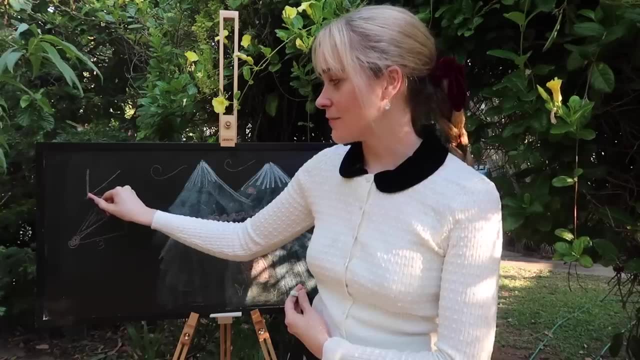 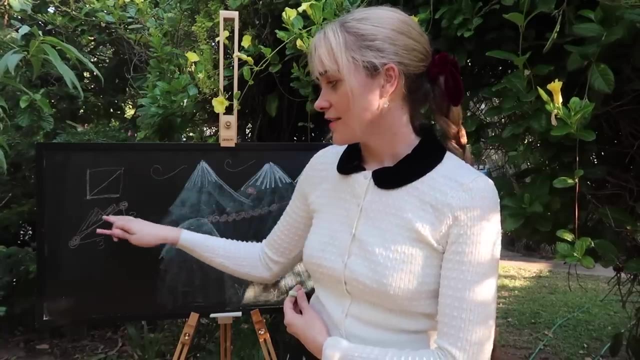 pebbles in this width. What it means for us is that our slope is exactly as tall as it is wide. It also means that it's exactly the same as this line here, because this line here is as tall as it is wide. So if everything is fine and our pebbles were a good little measuring stick, then 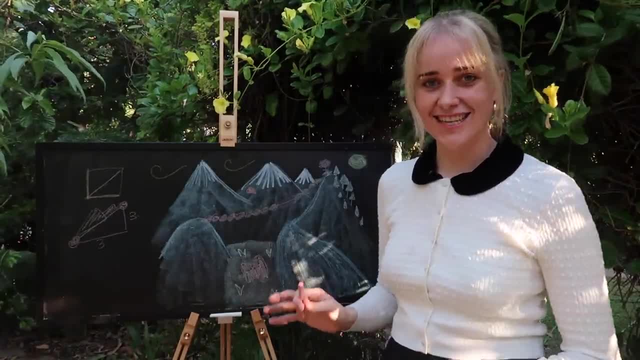 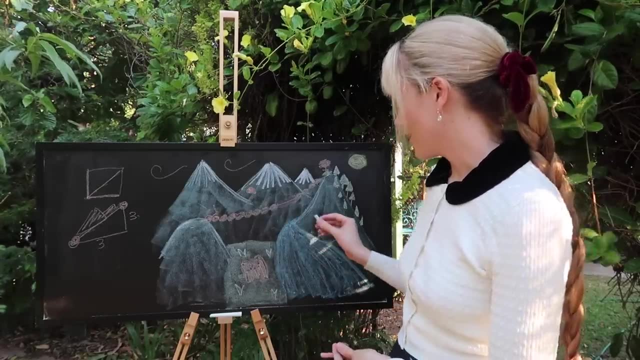 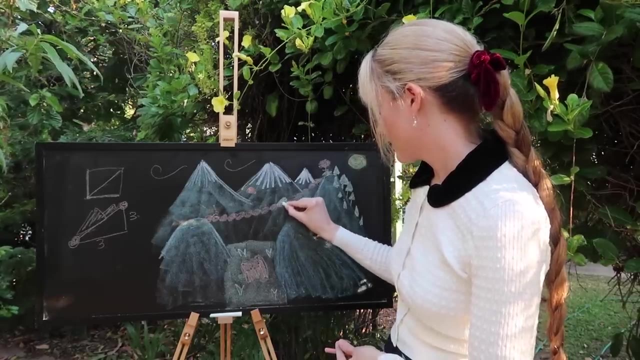 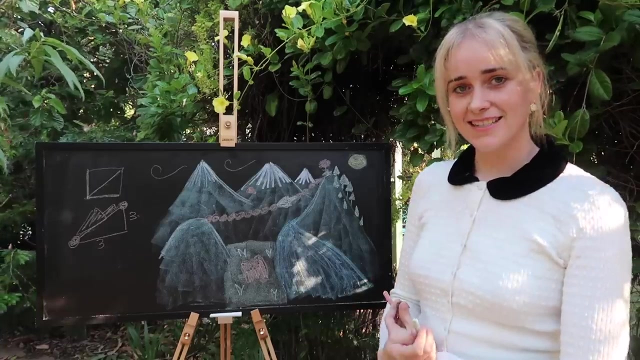 a little straight ramp here should be just steep enough for Bob to be able to handle with his shoes. So let's go ahead with it. Bob's pretty strong and he carries the tree down to the slope and puts it in here. So now a section of the bridge is our little tree, but it's pretty easy to cross. 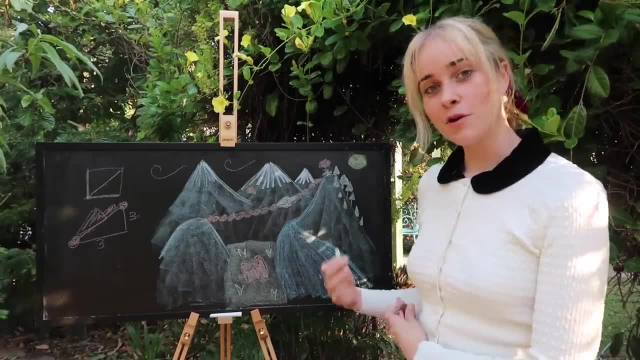 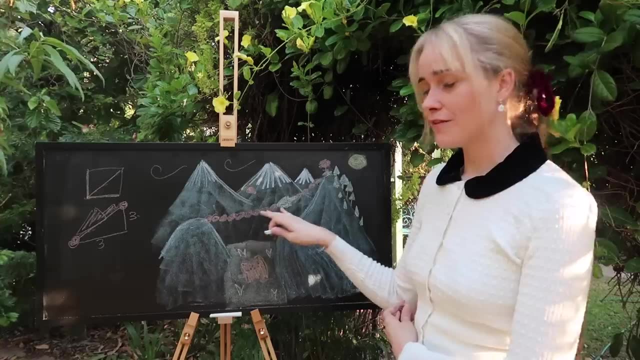 over. So if you're here to learn a thing or two about mathematics, then what we just did is differentiation. We had a curved line which is our entire bridge, and we found the slope at a point on our curved line just by zooming in on an. 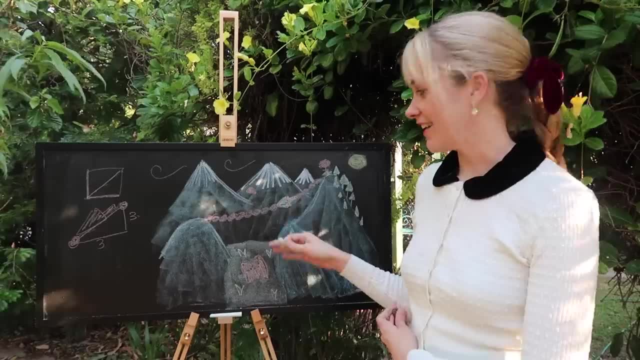 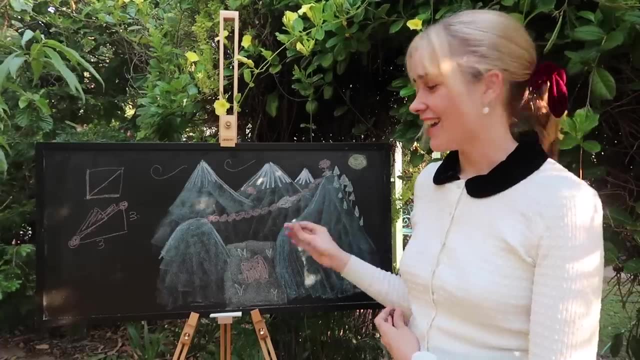 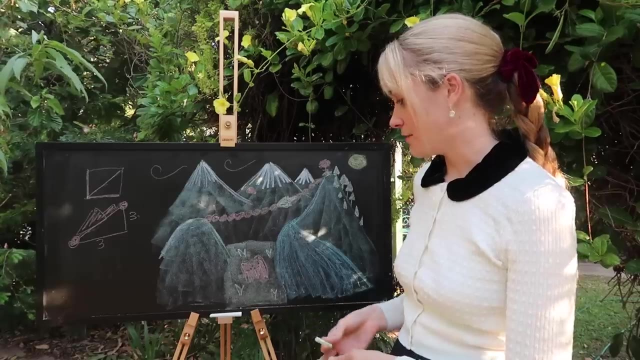 area of interest and treating that area as a straight line. In fact, in this case, we had a tree in there, so this section of our curve was treated as a straight line and we found the slope at that point. So let's keep going. Bob walks along the bridge and comes down into the meadow. Now what are in the? 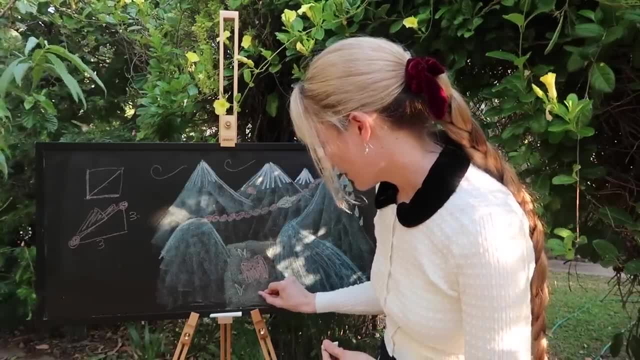 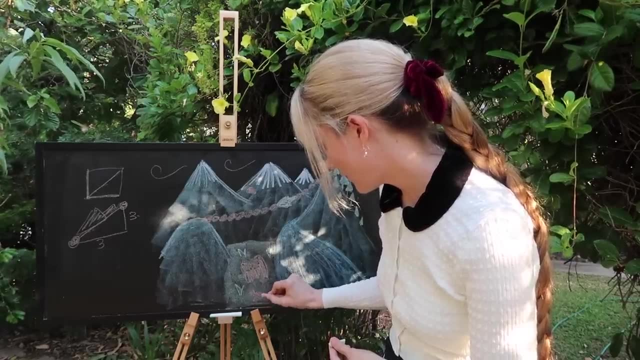 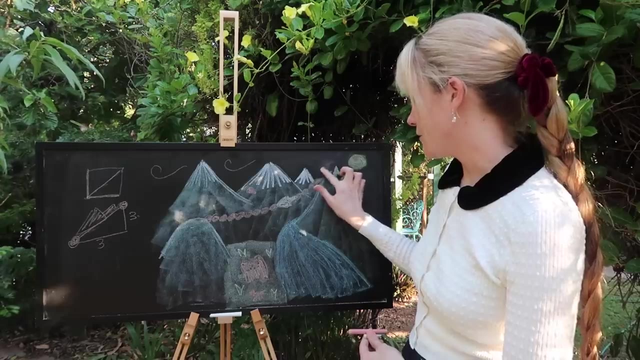 meadow are a couple of deer. Let's try and draw maybe one of those. on. A little head might be a bit hard to see. Some little legs Four- I don't know if deer have a tail. So Bob has gone down into the meadow and the first thing he notices 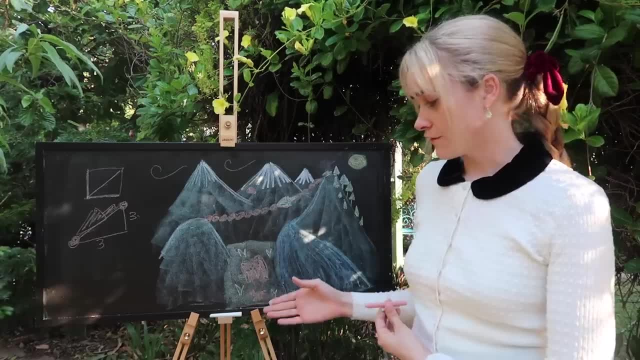 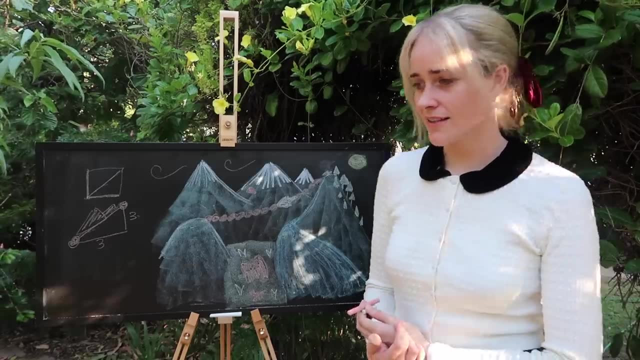 is that all the deer are alive. The piece of the bridge hasn't fallen directly onto any of them, so that's really good news. However, what he does start to get concerned about is the fact that quite a lot of the grass down here is now being. 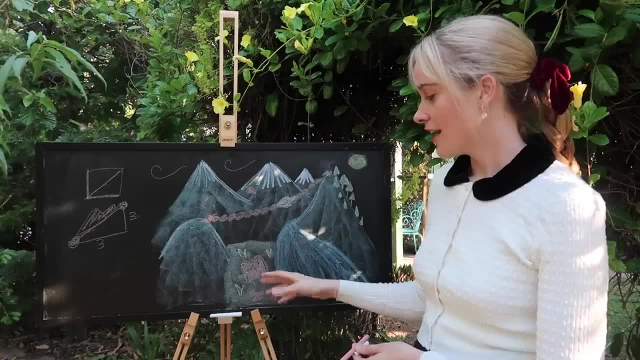 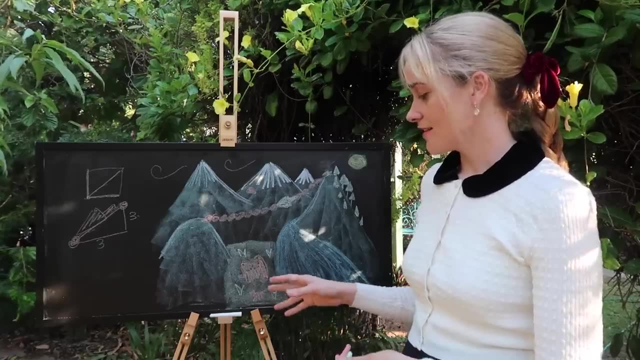 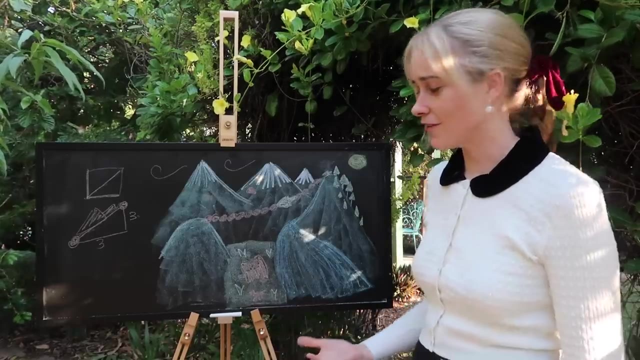 covered by this section of the bridge. Now it's kind of concerning because he knows there's not too much grass down here to begin with and he starts to think, you know, maybe with this grass gone and being inedible to the deer because it's covered in part of the bridge, 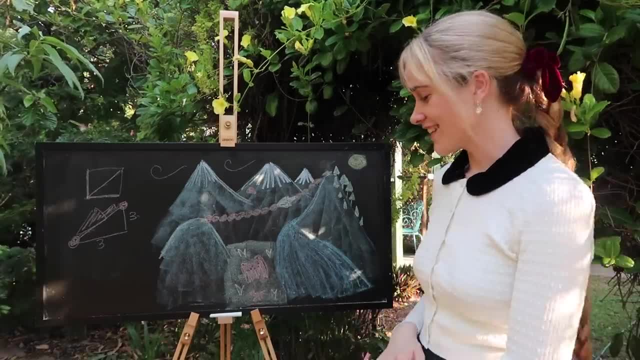 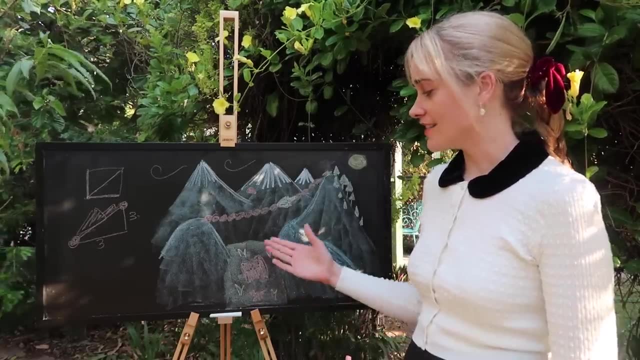 maybe the deer are going to run out of food. Bob knows exactly how much grass a single deer will go through in a season, so he knows how much grass is needed to be down here in this meadow. and because the meadow is just a rectangle, he knows 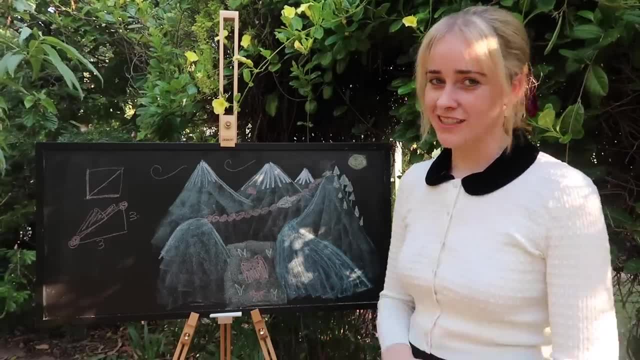 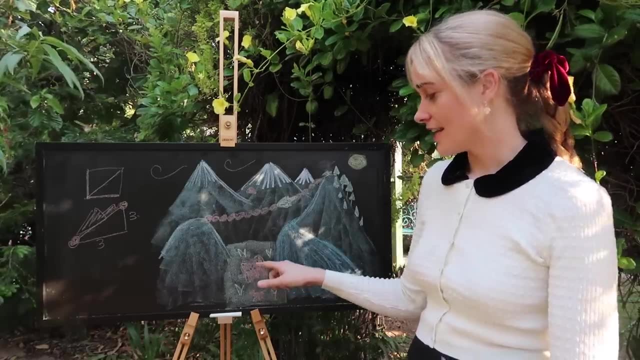 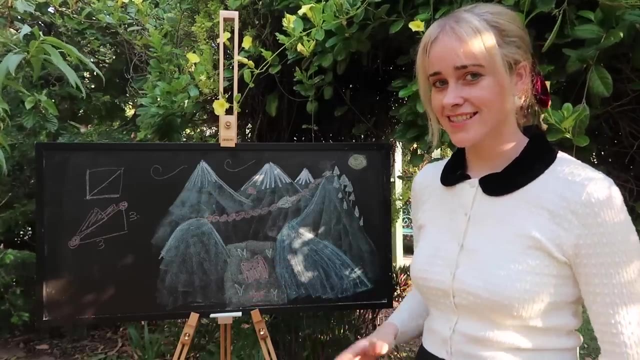 how much grass was there originally? What Bob really wants to know to make sure his little friends are going to be safe, is he wants to know how much of the area of the grass is now gone. He wants to subtract this amount from the total amount of grass and make sure it's still enough to 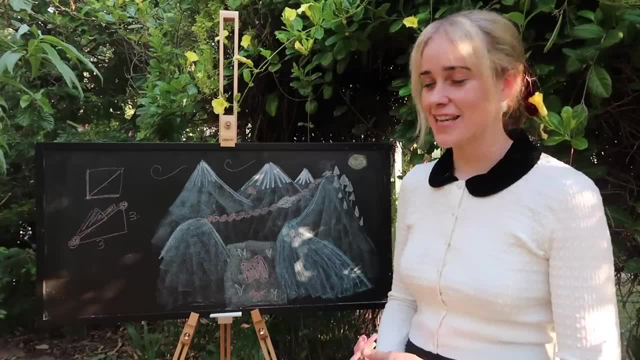 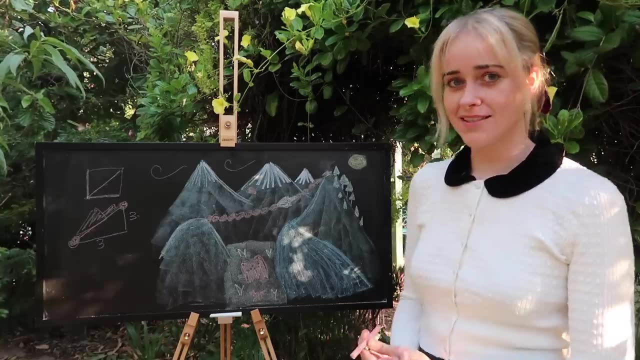 be able to feed the deer. If it turns out there isn't enough grass to keep them alive, Bob will probably have to call for help to move this section of the bridge out of their meadow or look for some other solution. So Bob gets down here. 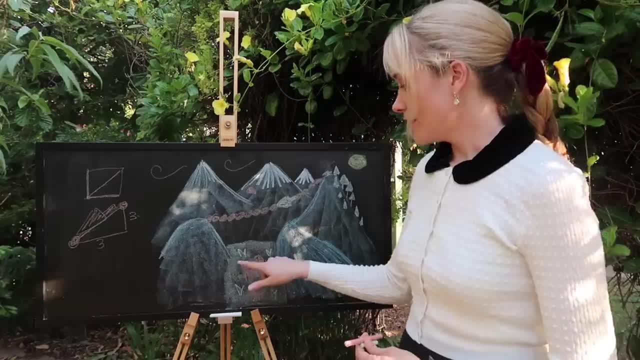 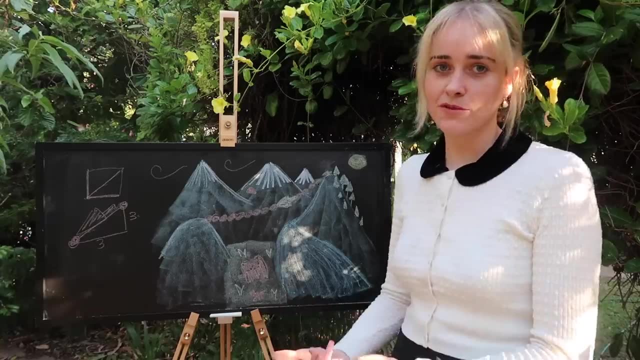 onto the meadow and he thinks: okay, I've got another problem. This part of the bridge that fell into the meadow is a very irregular shape. it's not a circle and it's not a square, otherwise I would be able to find its area quite easily. So he thinks: well, maybe I can approximate this as a circle. 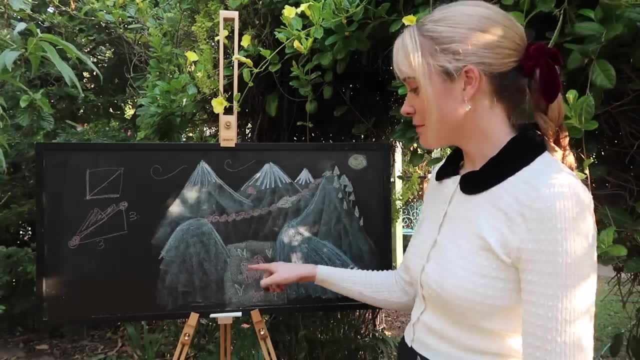 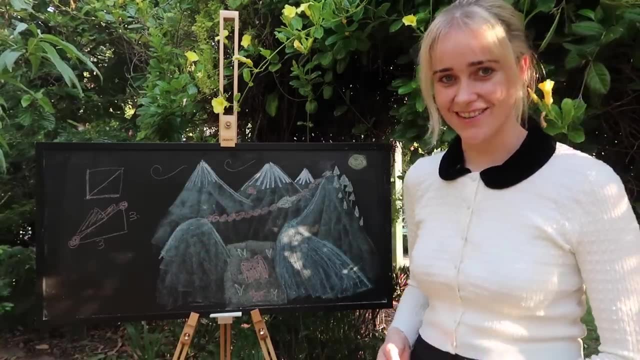 or I can use my trusty little pebble to try and measure how many circles would fit inside this irregular shape. Now I'm going to draw it up here to make it a bit easier for us to see. So this is the shape of the part of the bridge that's. 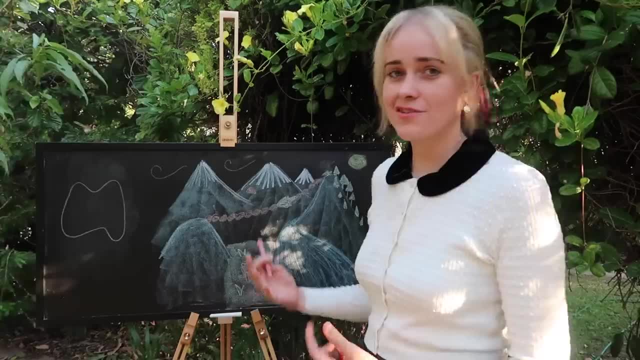 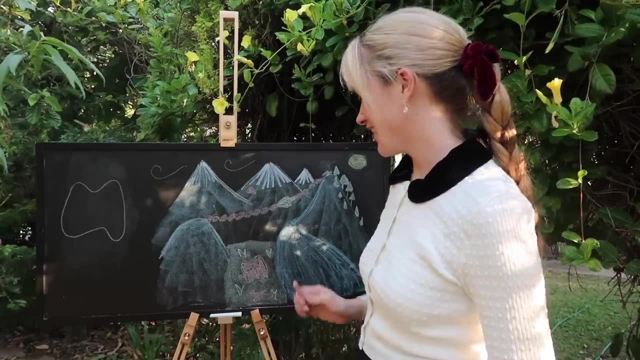 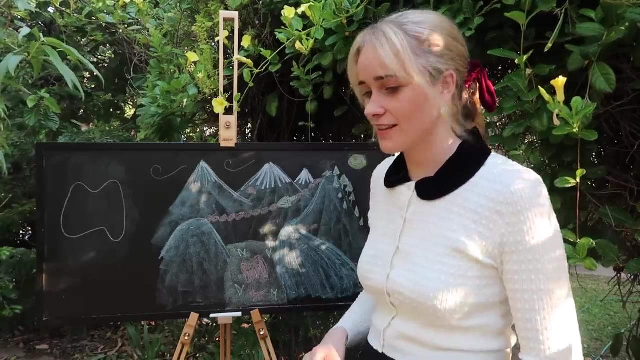 fallen into the meadow. Like I said, it's quite irregular because it's not just one log, it's a few sections of different logs that have fallen, Kind of looks like the shape of a strip of grass. So Bob thinks, okay, I all I know is is how to find the area of something like a pebble, if it's. 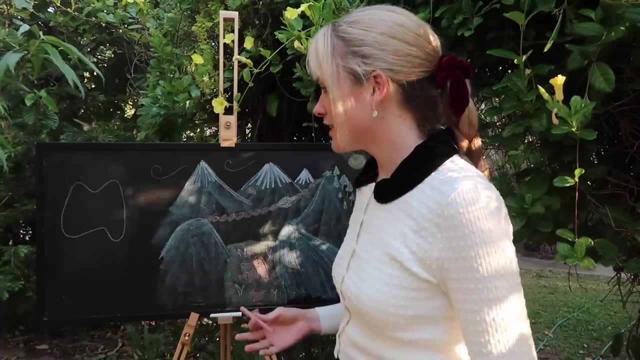 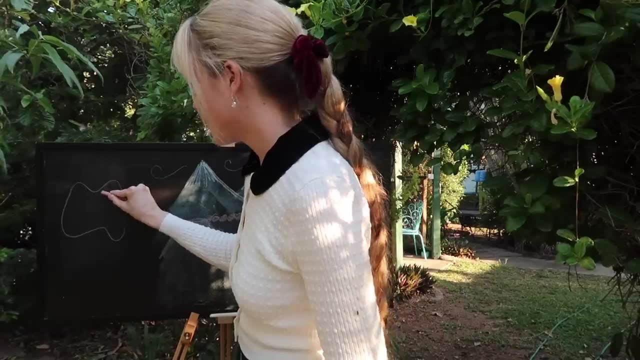 approximated to be perfectly round. So I've got a few of these pebbles. I can lay them out, I can get them from the riverbed and lay them along this shape and if I take my pebbles and lay them around, maybe I can lay them on top of. 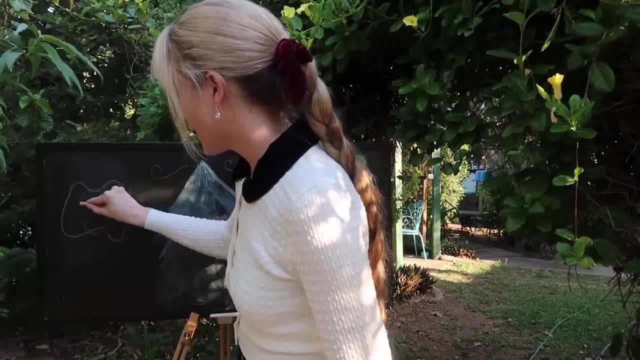 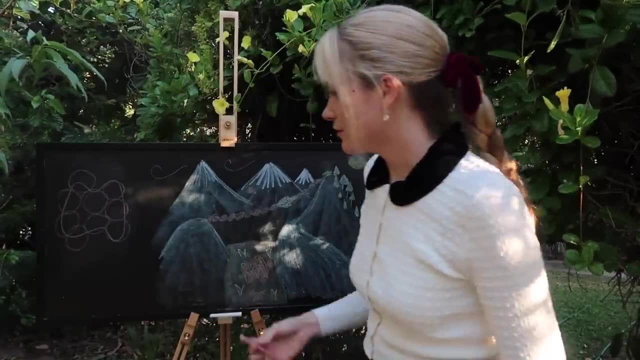 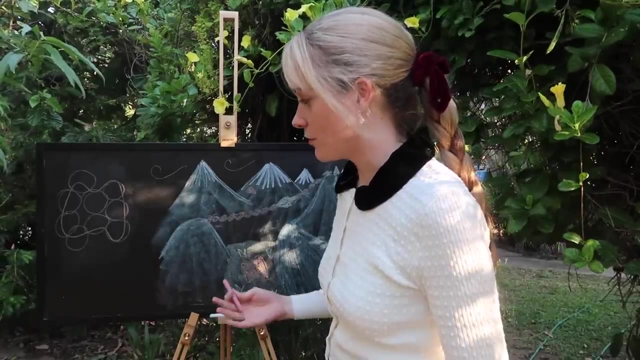 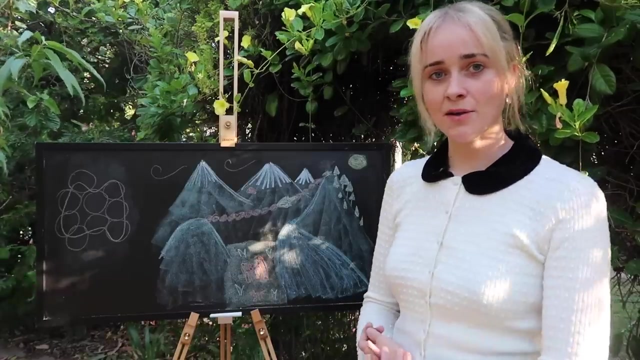 the shape and I can just sort of count how many fit into this shape. Now that's one way you could do it. you could count up the how many pebbles approximately equal the area of our unknown shape. Here we have one, two, three, four, five, six, seven, eight, nine pebbles. That might be an okay. 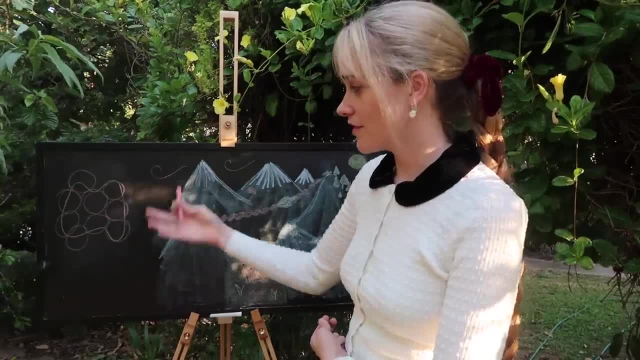 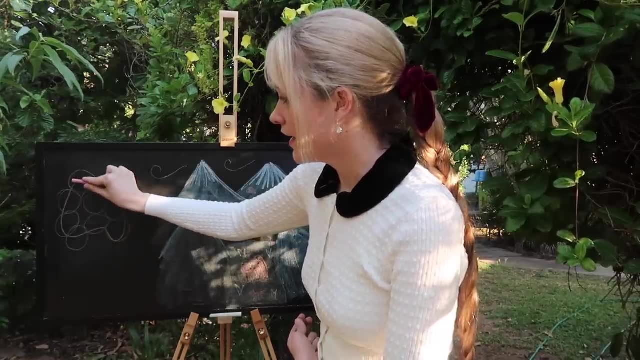 approximation. If you find the area of these nine pebbles, you can just say that's the area of the shape. But you know it's not perfect. we have some overhang here. so we're saying that this area is part of the shape when it isn't. We've got some gaps. 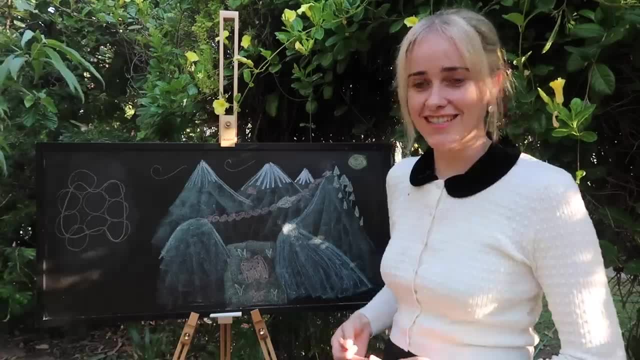 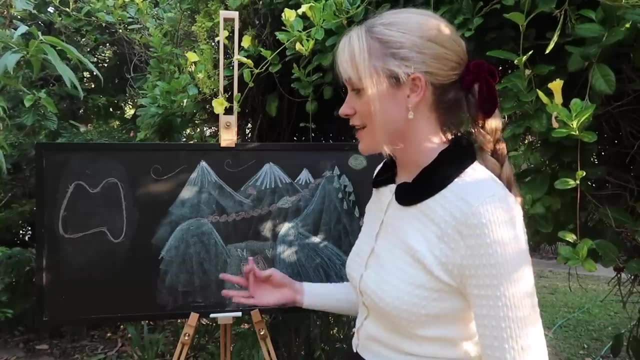 in here between the pebbles, because they don't perfectly fit together, and whilst this is an approximation, it's very far from perfect. So what Bob can do to get a better approximation of this area is to get some smaller pebbles. Now, if he lays, 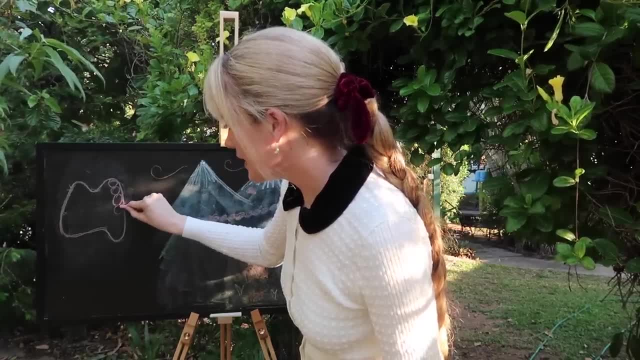 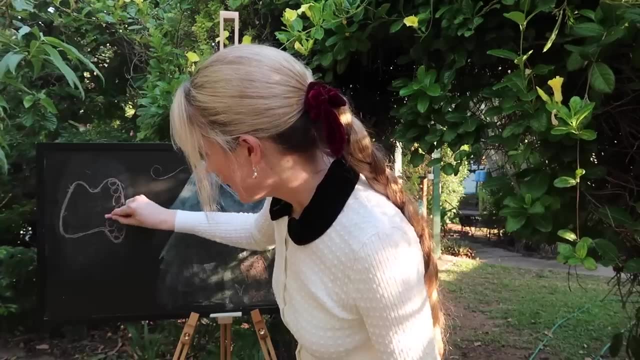 some smaller pebbles on here. there's going to be less of a gap between the pebbles, so less area. that's not being measured and when a pebble does overhang it doesn't go too far off our area. It's still not. 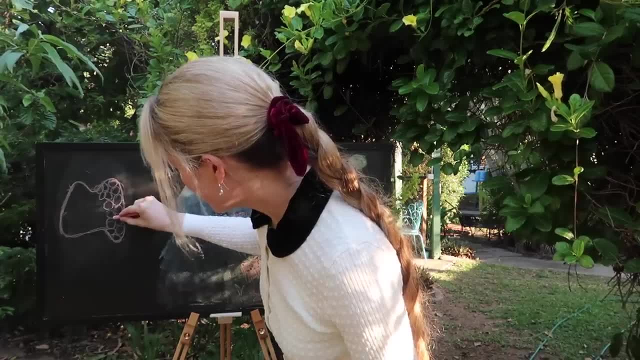 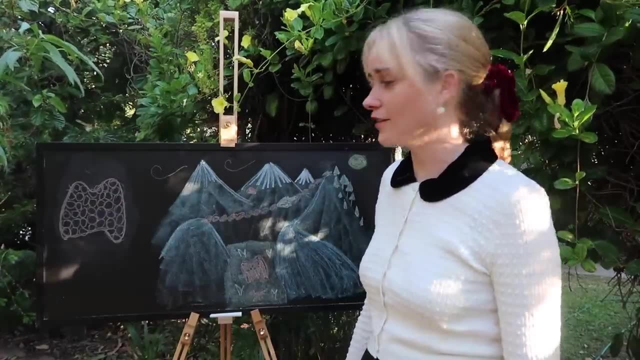 perfect. we still have a bit of overhang, we still have a bit of gap between our pebbles, but we're getting a bit better. So there we are. that's what our new measuring technique would look like. We've still got a bit of area in here. 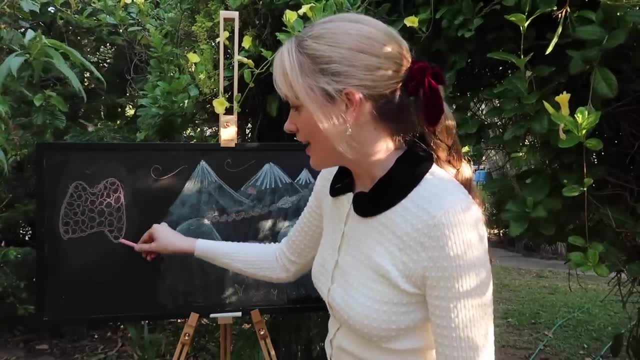 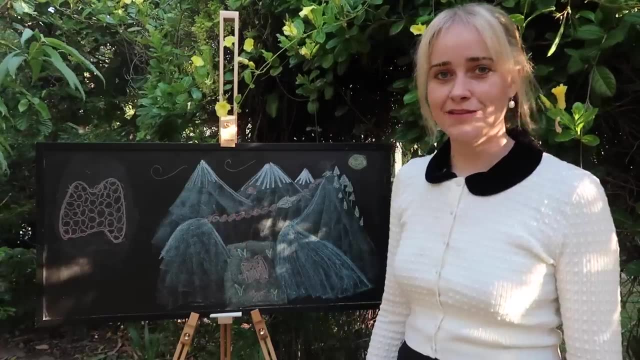 that's not being measured correctly by these pebbles. we've still got a tiny bit of overhang, but it's definitely a lot better than what we had before. You know, this might be good enough for some people, but Bob, he really cares about these deer and he doesn't want to take any chances with approximations He wants. 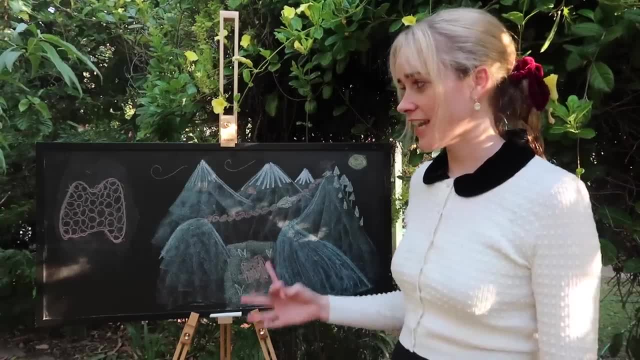 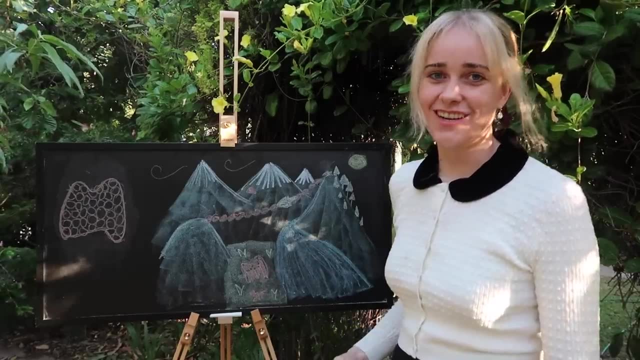 to know exactly. will these creatures be okay? Will they have enough grass? How much of their grass has been taken away from them by the bridge? We really want to know exactly. Okay, so this isn't good enough for Bob. He looks around him and 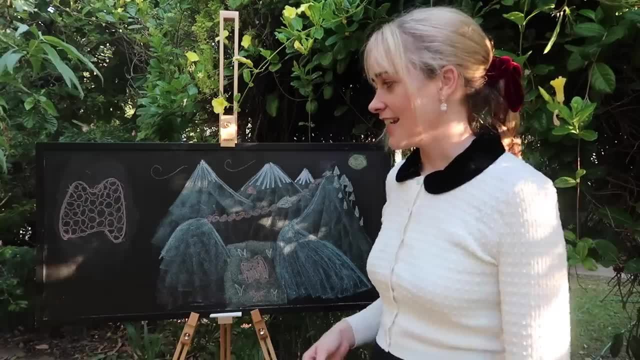 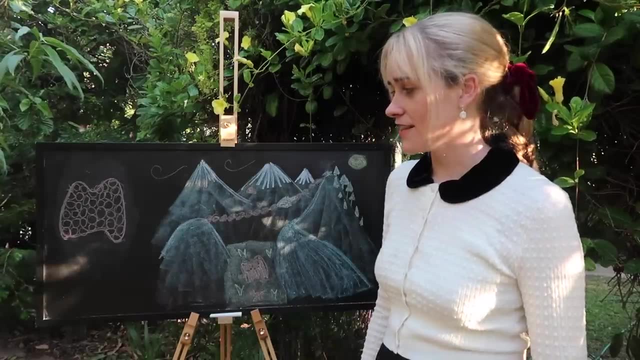 he sees the riverbed and he sees that it's made up of sand. Now, sand, I guess people. Bob knows that the smaller the size of the item he uses to approximate this area, the more accurate it's going to be. so he thinks to himself, you know. 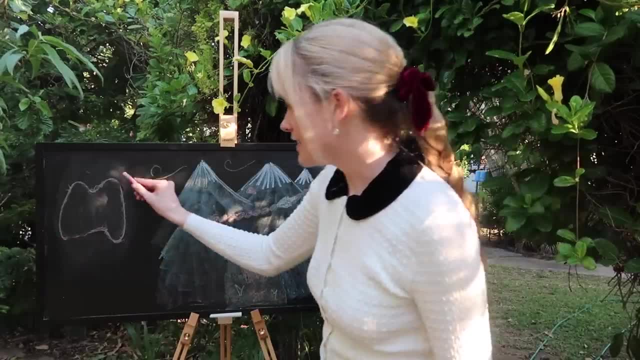 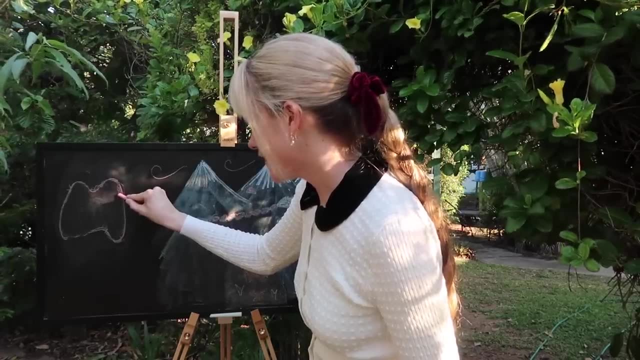 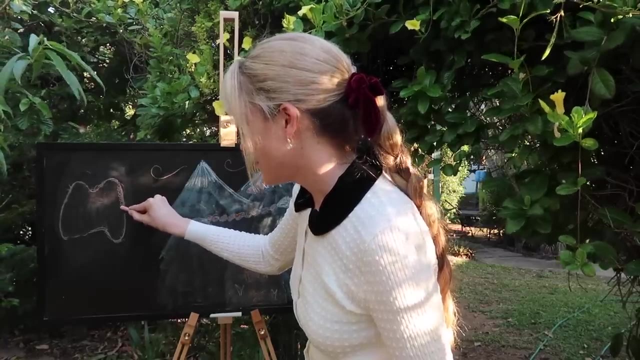 it's worth it. I'm going to get the sand. Bob lays individual grains of sand in little columns down the shape and he has to count exactly how many grains of sand he's placed. He knows the area of each grain of sand because they're perfectly. 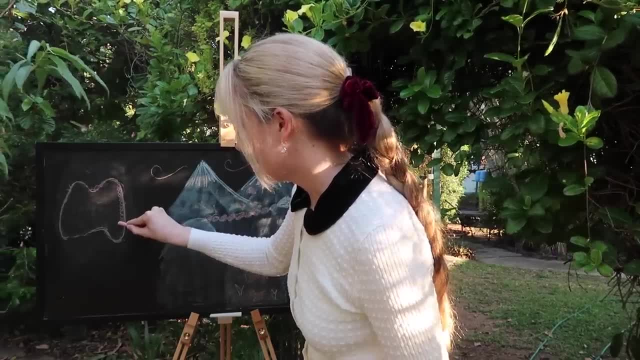 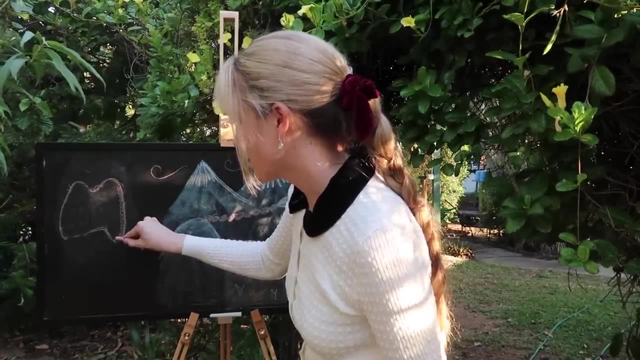 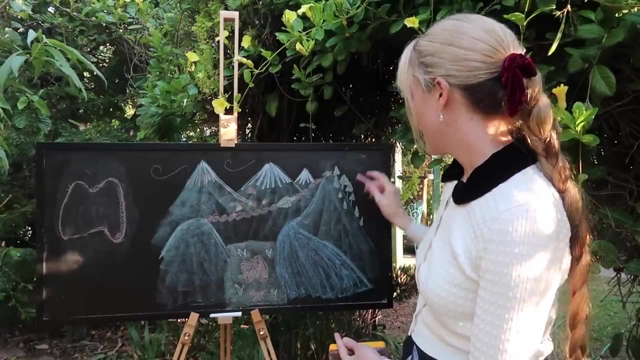 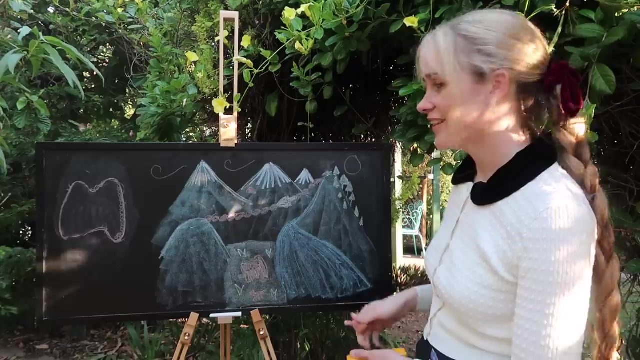 round grains of sand. He takes his time to lay them out, one by one, grain by grain, along the shape. It takes so long for him to do this that while he's laying them down, it's no longer day, It turns to night, and then it turns to day again, and then it turns to 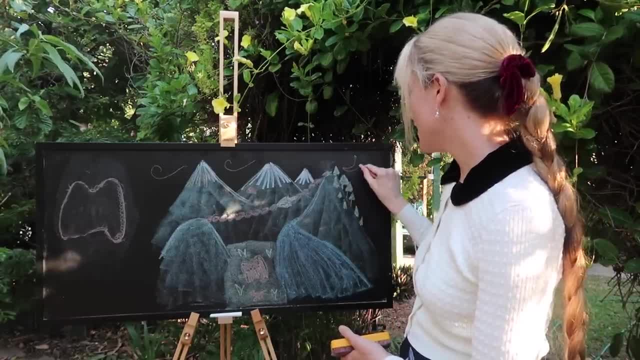 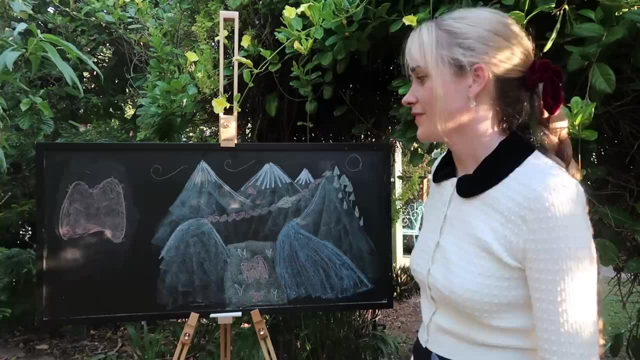 night. But Bob keeps going because he is really dedicated to these creatures and he wants to know exactly what's going on. He wants to know exactly what's going on. He wants to know exactly what's going on. He wants to do what he can to be as accurate as possible. A couple of days later, we are 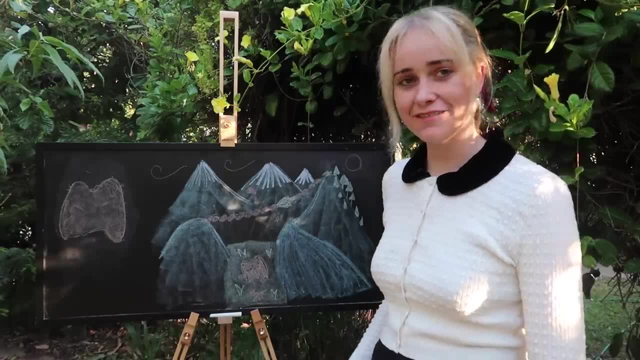 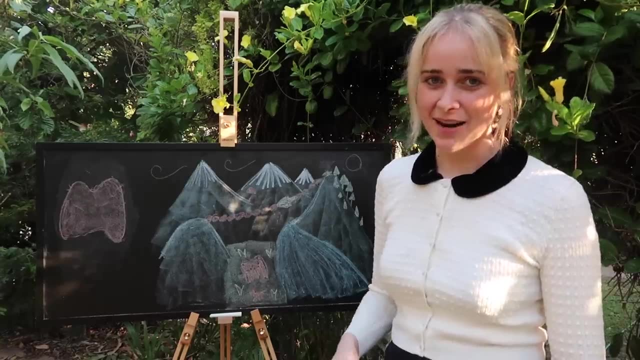 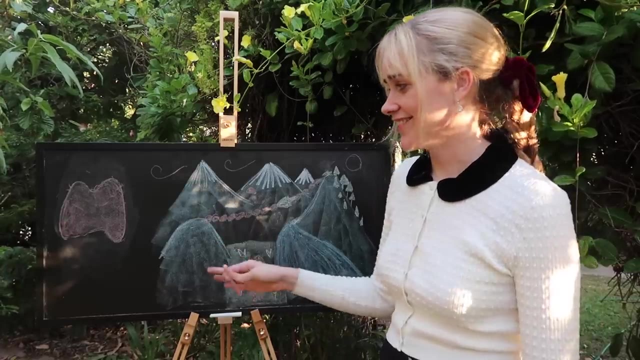 all done. It's back to sun and we've completely filled our shape with grains of sand. If you asked Bob how many grains of sand he laid down on that shape, he might say it seemed like an infinite number, but we were just getting very close to infinity. There's certainly hundreds of thousands of little grains. 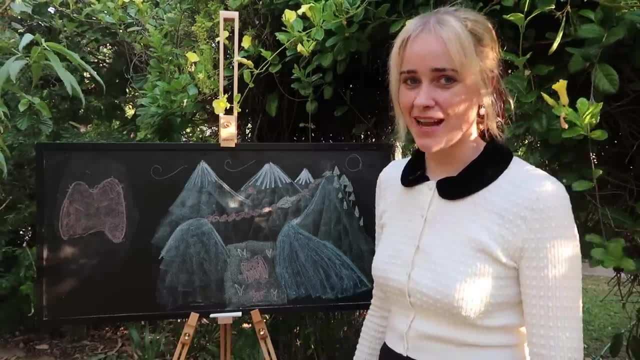 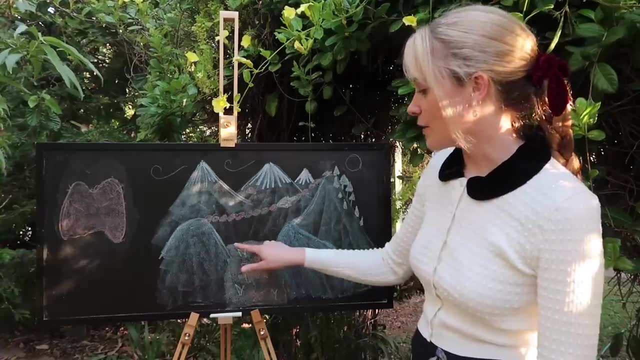 of sand on that shape. But the good news is that Bob has an almost perfect knowledge of the area of this shape here. So he pulls out his notepad, he works out the area of the original garden, he subtracts his now known area.